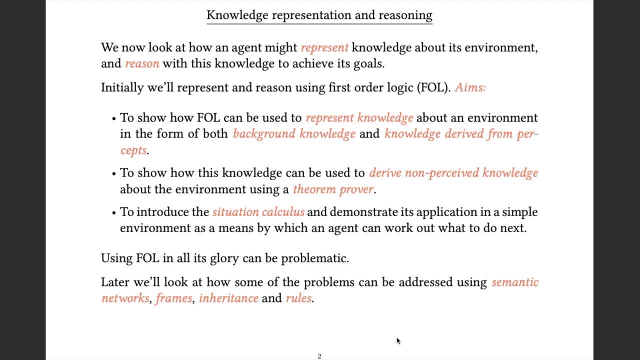 operating within some environment might need to have. One of the fundamental requirements for that architecture was to be able to represent certain kinds of knowledge about the environment and to reason with that knowledge in particular ways. So now I want to talk a bit about how one represents knowledge. 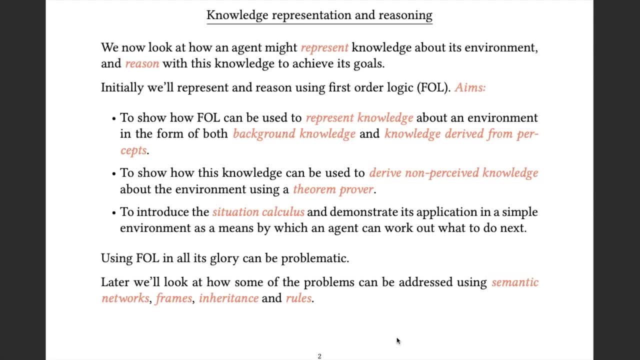 of the kind that was identified back there and, in particular, background knowledge and knowledge that's derived from our agent's percepts. I also want to talk a little about how, once we have a representation of knowledge, we might actually go about deriving new, non-perceived knowledge using a theorem proof. Initially, I'm going to do this using first-order. 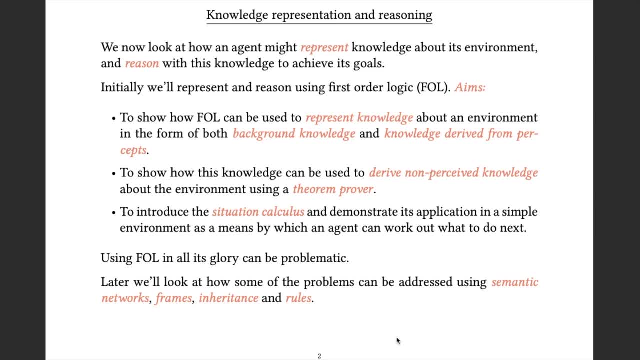 logic. Using first-order logic means we have a theorem prover. In fact, there are several industrial strength theorem provers for first-order logic. What's a little more problematic, perhaps, is to come up with some kind of systematic way of writing knowledge down in the format. 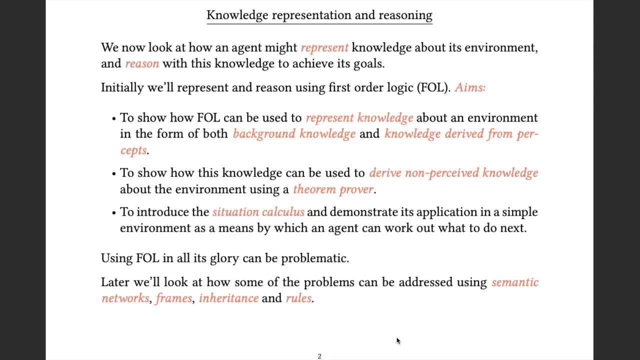 of first-order logic, I'm going to introduce one way of doing that which is called the situation calculus. First-order logic as a means in general of knowledge, representation and reasoning does have its drawbacks and, as a result, there are a whole bunch of alternative. 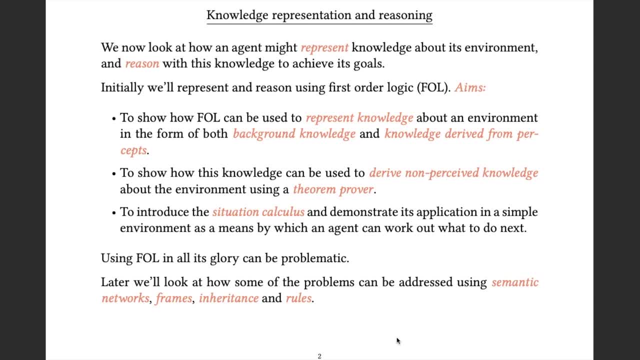 complementary ways of doing knowledge, representation and reasoning that have been built up over the years, Towards the end, in fact, probably in a separate video I'll talk a bit about semantic networks, frames, inheritance and rules, But these tend to be very first-order, logic-like and, in fact, can quite often be a little bit more complex than what we're used to seeing in the first-order logic. First-order logic can be a little bit more complex than what we're used to seeing in the first-order logic, But these tend to be a little bit more complex than what we're used to seeing in the first-order. 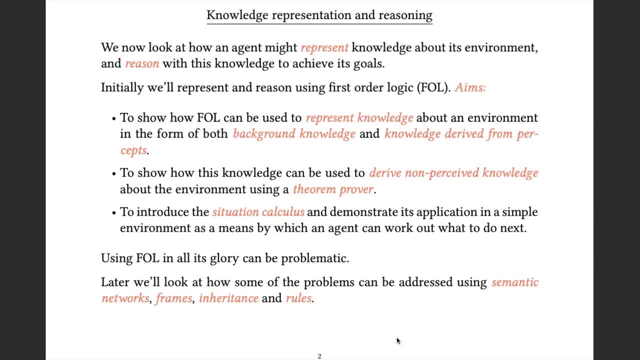 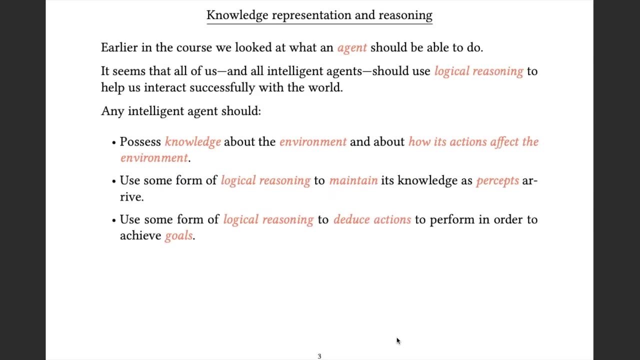 logic. First-order logic can be formally described as more limited versions of first-order logic, either in the sense of how you're allowed to do the representation or in the sense of how the reasoning process operates. Be more specific about the kinds of knowledge that need to be. 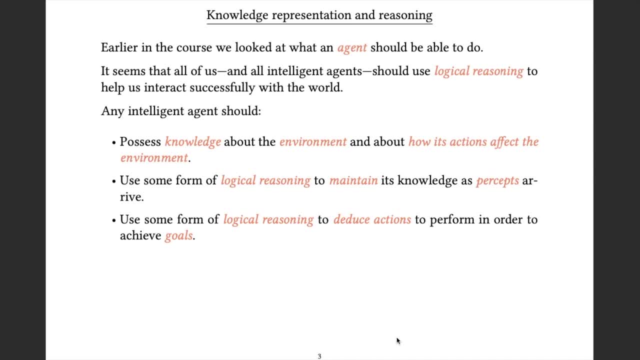 represented and the kinds of reasoning that an agent needs to be capable of. within the standard kind of architecture that I introduced, I specifically identified the need to represent knowledge about how the agent's environment works and, in particular, the need to represent knowledge that describes the environment and the way in which actions 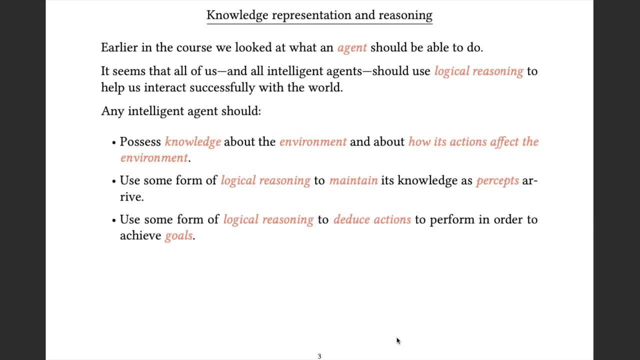 performed by the agent will affect the environment. I also identified the idea that one might need to use logical reasoning to update and maintain knowledge about the environment as precepts arrive, And I identified the need to perform some kind of logical reasoning to deduce actions to perform in order to get to goals. Now, hopefully you can see that there is a natural 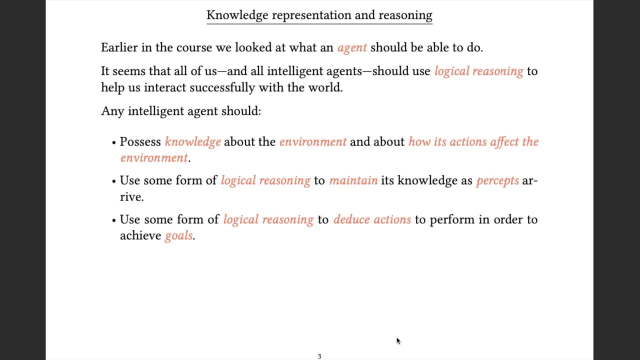 progression here, And that natural progression is based on the idea that an awful lot in classical artificial intelligence is cast as some kind of logical progression And that natural progression is based on the idea that an awful lot in classical artificial intelligence is cast as some kind of. 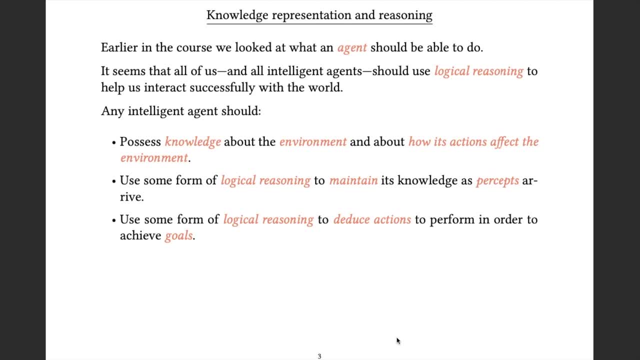 search problem, which involves finding sequences of actions to get an agent where it wants to go. But the level of complexity used to describe and to implement those search problems can vary quite wildly. We started with the most basic possible context and came up with a star and more intelligent versions of search. Now we're building on that and allowing 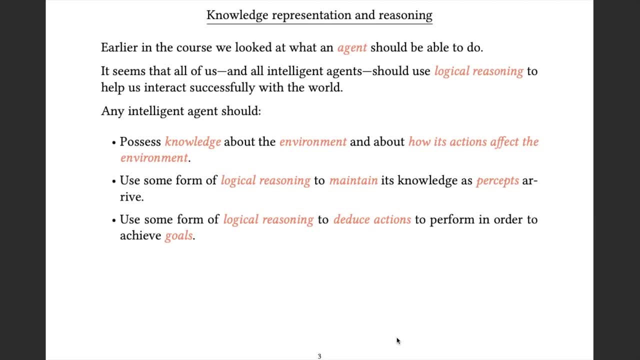 a language for the description of our knowledge that's much more flexible than the one we started with and has a consequently more interesting and capable method for doing logical inference, But the underlying idea is very similar. we're just introducing more and more flexibility, Now that 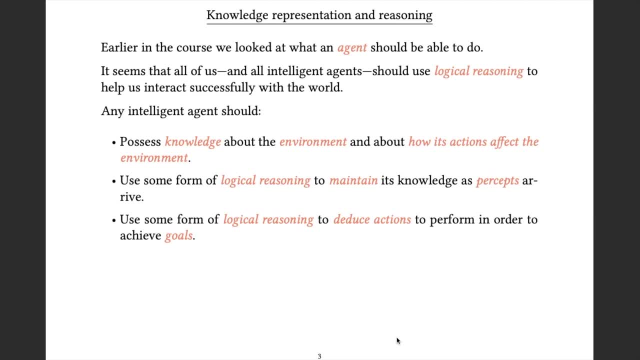 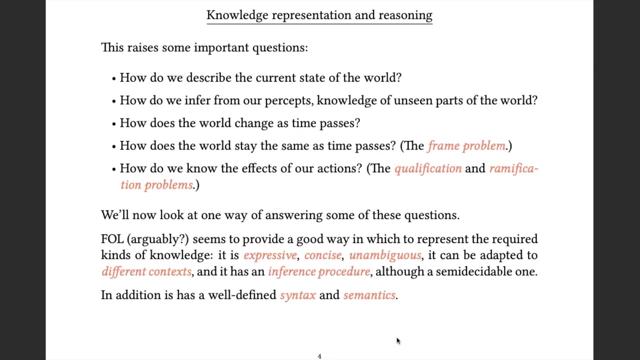 flexibility here is going to turn out actually to come with problems of its own, and the next subject, after I've spoken about knowledge, representation and reasoning, will try and address some of those issues by looking at specific algorithms for constructing plans. So now we have some specific kinds of problem. 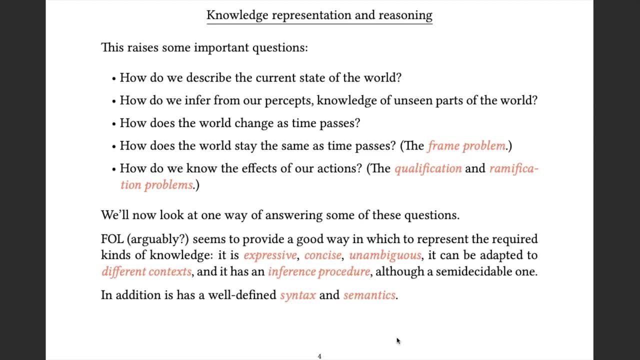 that we want to solve. We want to know how to represent our agent's knowledge about its current state of the world. We need to be able to infer things about unseen parts of the world And, importantly, we need to model the way in which the world changes as time. 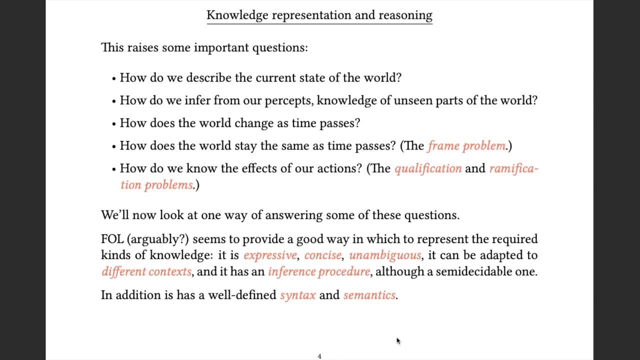 passes, either independently of our agent's actions or as a result of our agent's actions. And, equally importantly, we need to be able to model the way in which the world stays the same as time passes. A final point here is that if we look at these, these bullet points, time seems to 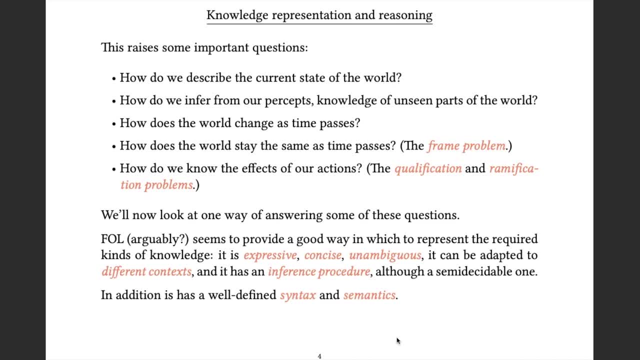 be particularly significant and clearly in the lives of many intelligent agents, time is indeed significant. Now, one result of that has been that in the methods we're going to look at, time takes a key, time plays a key role and indeed in the wider area of knowledge, representation and reasoning. 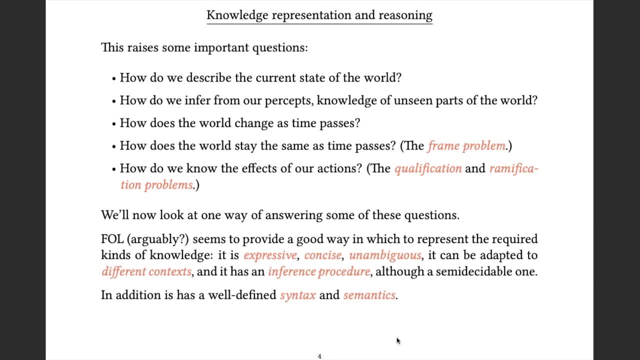 time takes a key role in the way that we think about the world, So we need to be able to control it in a sudden is one way or another. Similarly, time takes a key role in our understanding of the world. In our model. we have a number of different methods we may want to take to 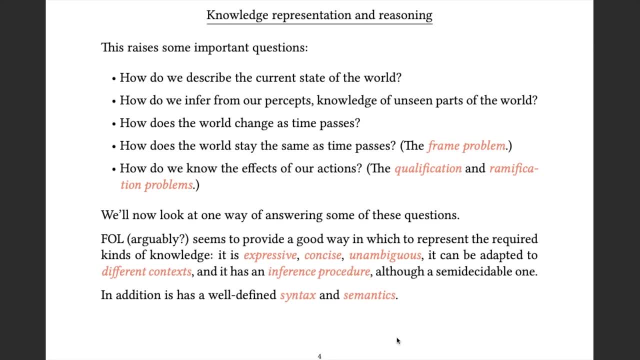 understand the world to be more clean and secure. The field of time. lemme demonstrate this real quick. First order: logic seems at first glance, and with some deeper examination, to be a good way of doing this, because it has all of the characteristics we want from a form ofシ. 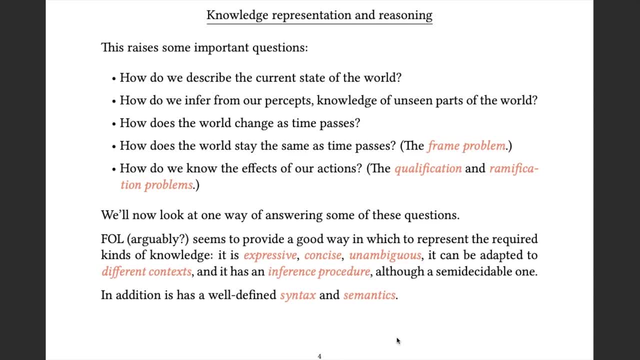 dub Difference in thrive logica. It's concise, it's not unduly worthy, it is non-ambiguous, you can adapt it to many different contexts and it has an inference procedure, Although the inference procedure for first-order logic is semi-decidable. 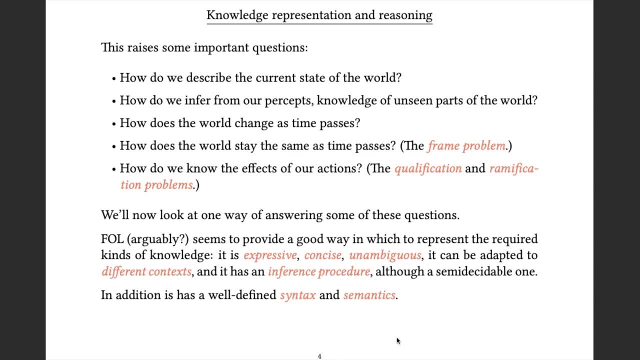 there is no algorithm that guarantees to take any first-order logical formula and tell you whether or not it is valid and always give you the correct answer and always terminate. But a lot of the time we can run an inference procedure on a first-order logical. 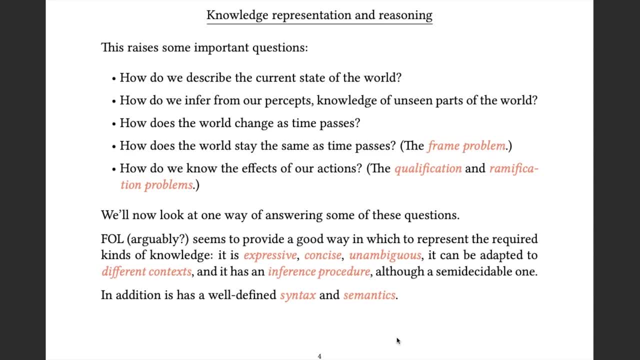 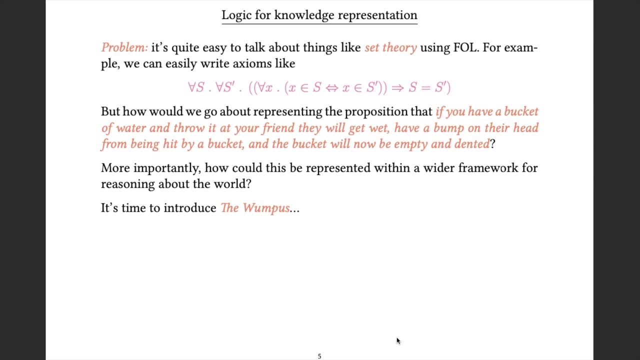 formula and get an answer. Finally, first-order logic has a well-defined syntax and semantics which is arguably just as important as its other desirable characteristics. But that's not to say that it's necessarily straightforward to make progress here. If you have something mathematical and cleanly and well-defined, like set theory, you can easily 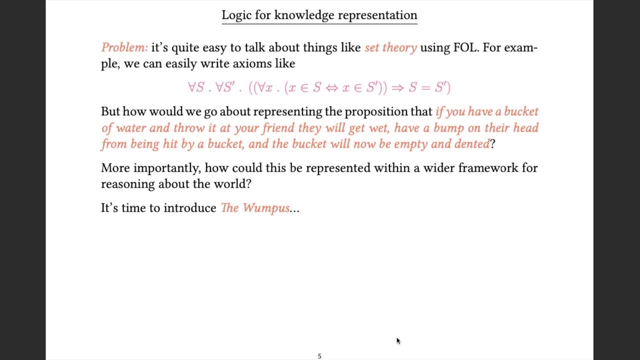 write little chunks of first-order logic that describe how your world works, in this case the world of set theory. And here I just have an example that says: if you've got a pair of sets, then if, for all x, x is in the first set, if, and only if, it's in the second. 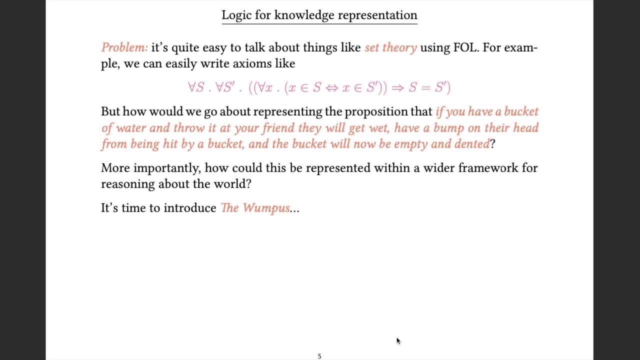 then the two sets are the same. Now, in fact, that's just a quick and dirty example that is being used specifically for the sake of having an example. It turns out that defining sets within first-order logic has its own bunch of pitfalls, but I'm not going to go into that. 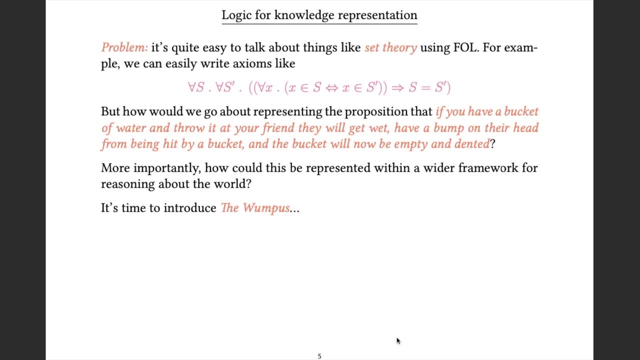 Because the point that I really want to make here is that, while it's easy enough to try and write knowledge down regarding things like sets or natural numbers or various other parts of mathematics- if you want to take a more artificial intelligence oriented example- like if you have a bucket of water and throw it at- 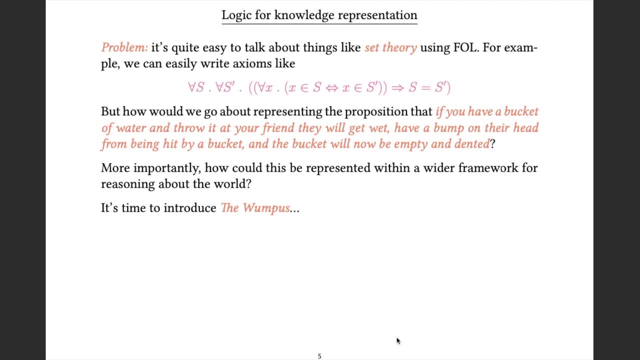 your friend. they will get wet, have a bump on their head from being hit by a bucket, and the bucket will now be empty and dented. Well, it's a bit trickier to see how you might go about representing a piece of knowledge like that using first-order logic. So we need to look at how knowledge of the 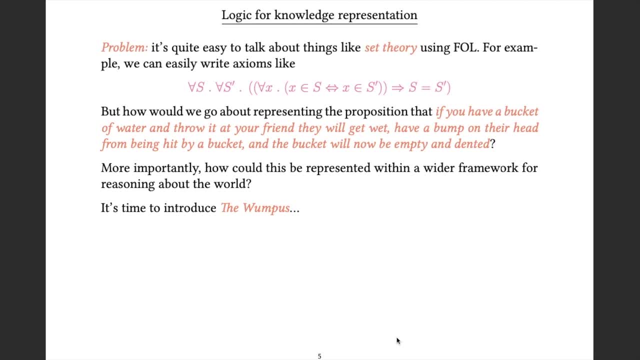 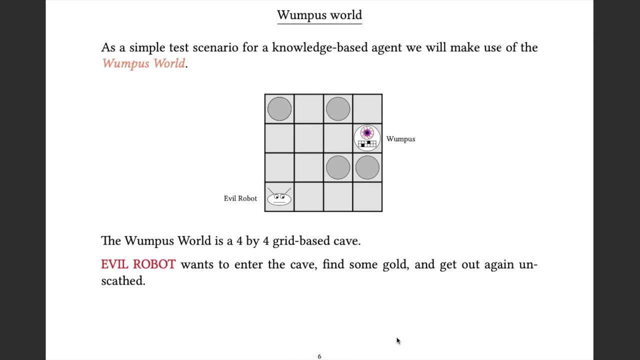 kind that might need to be manipulated by an intelligent agent in an environment can actually be represented using first-order logic, And in order to do that, I need to talk about the wampus Now. wampus world is a classical AI test case used for, amongst other things, talking about: 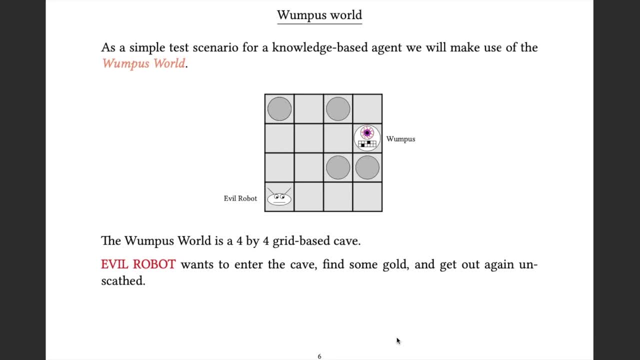 knowledge, representation and reasoning. The wampus world is a 4x4 cave that's laid out on a grid. The cave has a wampus in it and it also has some gold not shown here. And if we want to program our intelligent agent, namely Evil Robot, to play the 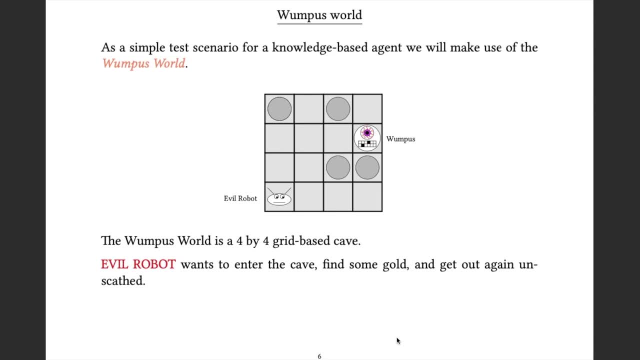 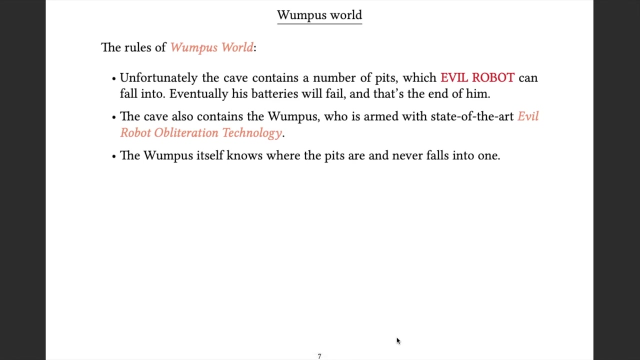 Wampus World game. the idea is that he should be able to enter the cave, navigate around inside the cave and retrieve some gold, then find his way back to the entrance point and leave the cave again. But, as you could probably guess, there are various things about the cave that will try and thwart Evil. 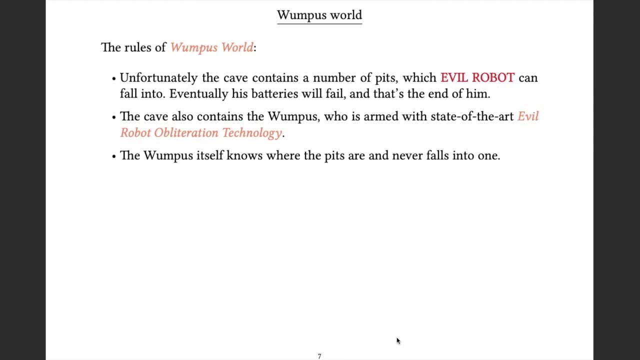 Robot's efforts. Firstly, the cave has a number of pits in it. If Evil Robot falls into a pit, then eventually his batteries fail and he will die. The cave also contains the Wampus, who is armed with Evil Robot obliteration technology. So 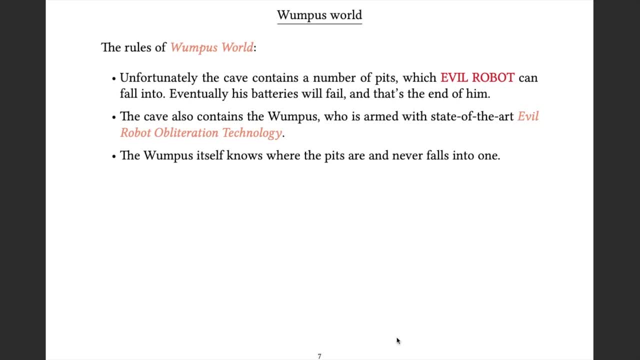 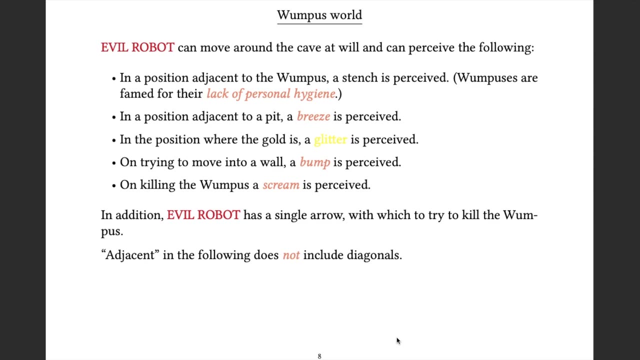 Evil Robot wants to avoid the place where the Wampus is, because if he goes there he will also die, And the Wampus itself knows where the pits are and never falls into them. And we have some more. While Evil Robot is moving around, he can perceive various things. First, if Evil Robot is adjacent, 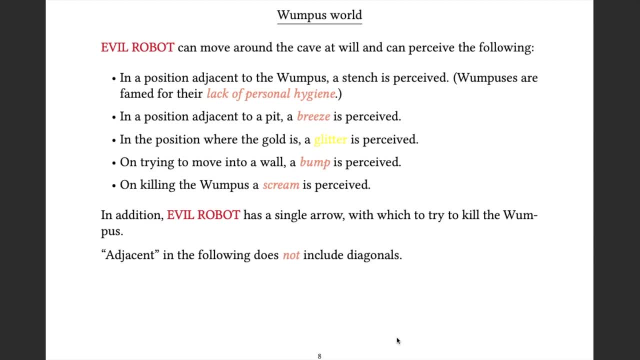 to the Wampus. and adjacent here doesn't include diagonals, it's just adjacent vertically or horizontally, then Evil Robot will die. Well, Wampuses are famed for their lack of personal hygiene and they have ten arms each and great big armpits, and they've never heard of underarm deodorant. So when 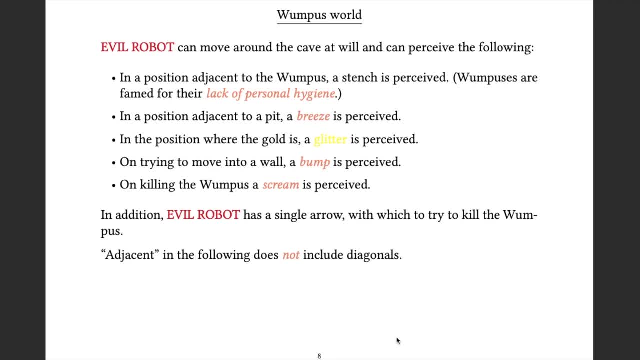 Evil Robot is adjacent to a Wampus, a stench is perceived. In addition, when Evil Robot is in a position adjacent to a pit, a breeze is perceived. I've never found an explanation for why pits make breezes, but that's the way it works. 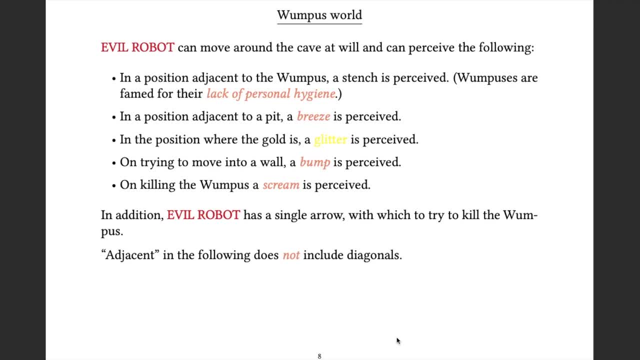 If Evil Robot is in the position where the gold is, then he perceives a glitter, and if he tries to move into a wall, then he perceives a bump. Now, as an extra part of the game, Evil Robot wants to kill the Wampus. He therefore carries a single. 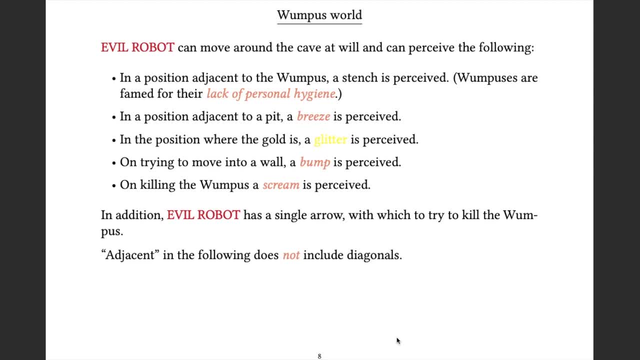 arrow which he can shoot And he will shoot it in whichever direction he's currently pointing and he will know if he has killed the Wampus because he's not going to die. If he manages to kill the Wampus by shooting it with the arrow, then he will receive a. 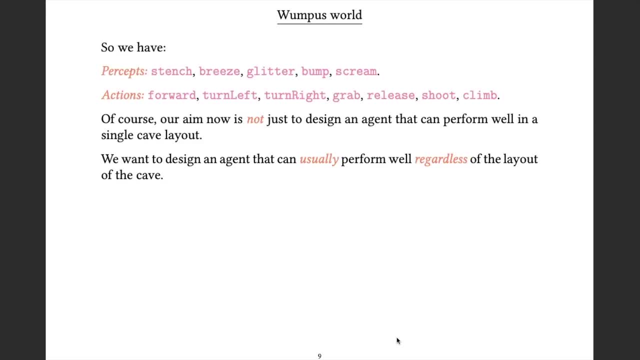 scream. So, considering Evil Robot as an intelligent agent, now we have some perceptions that Evil Robot can make and we have some actions that Evil Robot can perform. While moving around the cave, he can perceive a stench, a breeze, a glitter, a bump or a scream. And, in order, 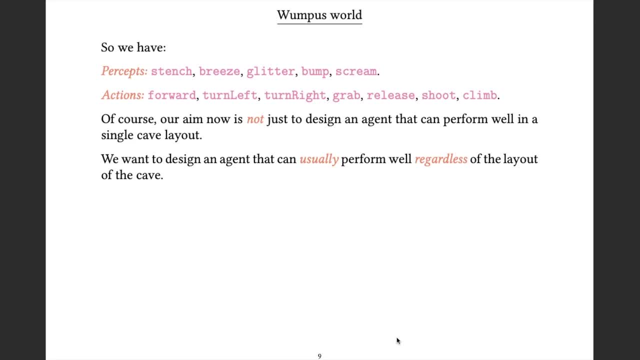 to solve this problem. he can move forward and he can shoot. He can shoot a whip, he can shoot a squash, he can shoot a knife-sm. Tiger's Keep. turn left by 90 degrees, turn right by 90 degrees. he can perform a grab which lets him try to pick up gold. he can perform a release which lets him drop the gold. 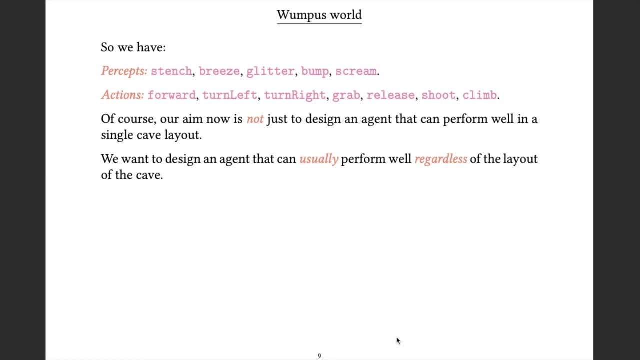 There's no particular reason in the game that he would want to do this, but we're including it as a possible to shoot the arrow in the direction he's pointing and he can do a climb, which is an attempt to get out of the cave. Now there is, of course, a key issue here. 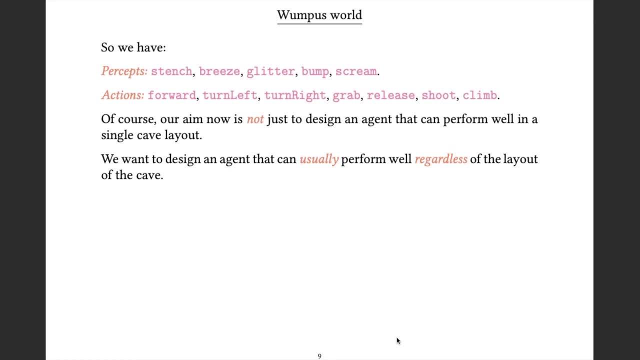 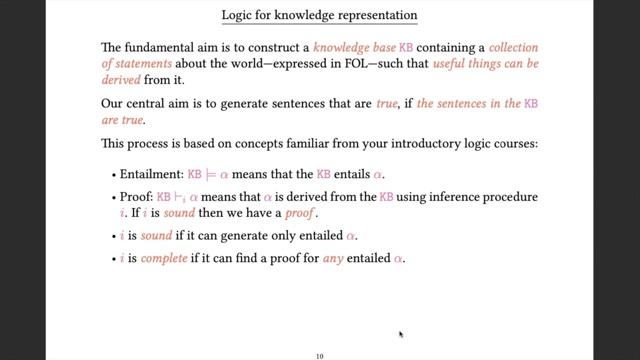 which is that we want to represent knowledge about this problem and perform inference with it in a way that allows Evil Robot to perform well, usually in arbitrary cave layouts, not just in a specific one of the kind that I illustrated on a slide. a couple of slides back. I need to start here by 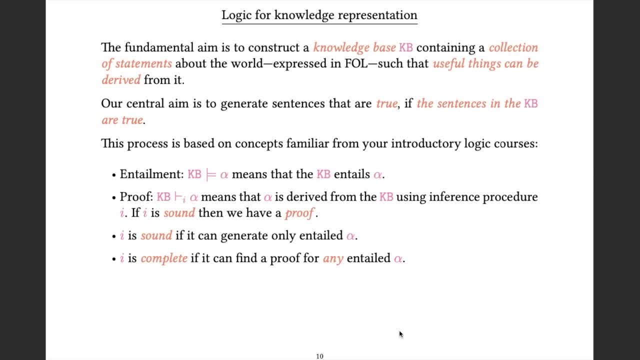 revisiting some of the underlying concepts that you met last term in the Logic and Proof and Prolog courses. The underlying idea here is to make a knowledge base. A knowledge base just contains a collection of statements about the world. In our case, we're going to start by expressing those statements in first. 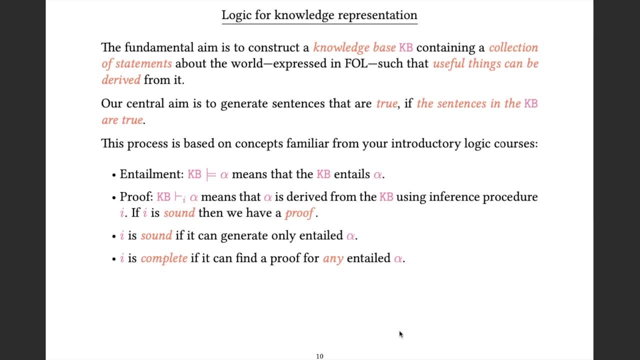 order logic and we want to represent them in such a way that we can derive useful things from them. But I just need to recap, really, what that last bit means, what it means to derive useful things from the knowledge base. That means, in essence, that we want to 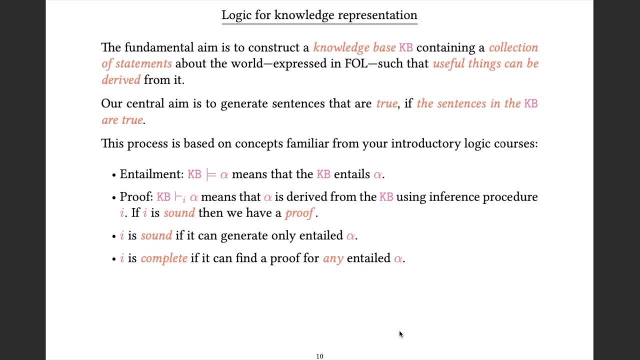 generate things that are true. if the sentences in the knowledge base are true- And you've seen this in logic and proof, because you've seen the idea of entailment- If you have a bunch of first order logical statements and you say that they entail a further. 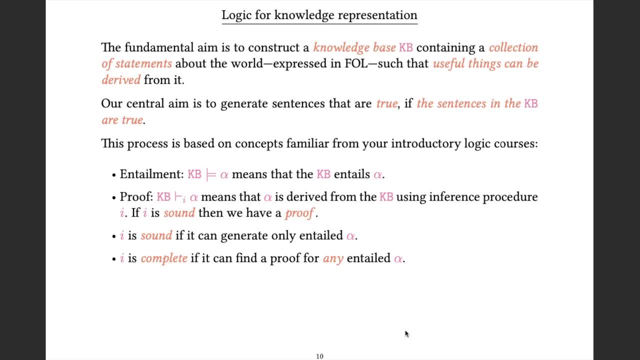 statement where, in our case, the collection is called KB. that's the knowledge base- and alpha- here is the thing that you're claiming is entailed. what this means is that any model that makes all of the statements in the knowledge base true also makes alpha true. 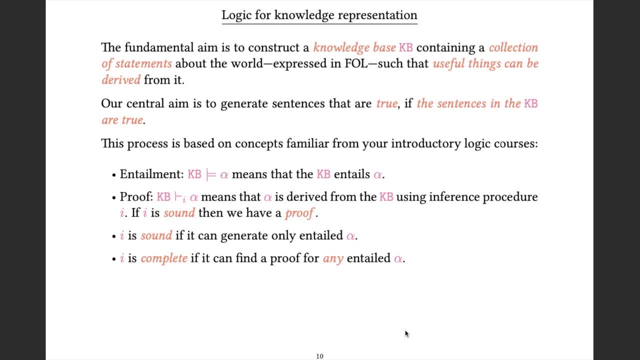 Now remember that a model just assigns actual functions and predicates to the function names and the predicate names that are in the knowledge base. It also assigns a particular set that acts as the universe, and functions have to map things in the universe to other things in the universe. 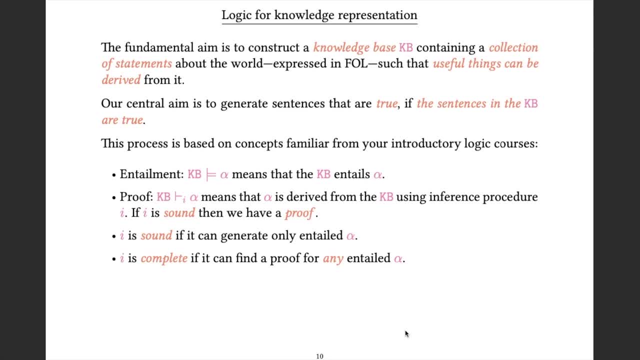 and predicates have to act on collections of things in that universe. But the key idea is that any way of doing that that results in all the statements in the knowledge base coming out as being true will also make the statement alpha true, The idea that alpha can be proved by some. 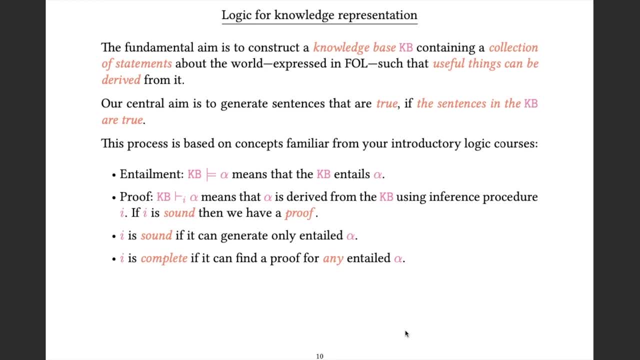 inference procedure i from the knowledge base, then we hope encapsulates the same kind of idea. This is a purely syntactic symbol shuffling procedure that gets you from the knowledge base to alpha, But in practice what we want is a sound and complete inference procedure, and that means well. 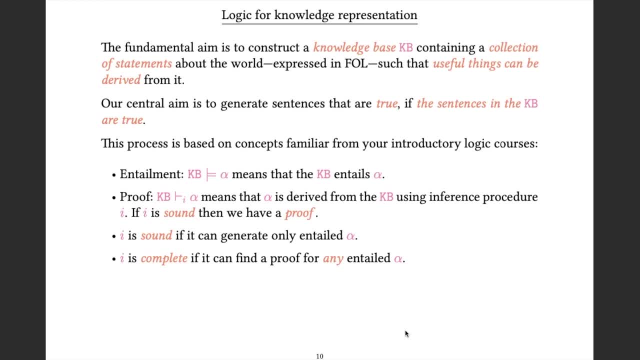 i is sound if this symbol shuffling mechanism can only lead you to alpha that are actually entailed from the knowledge base, and is complete if it can find a proof for any entailed alpha. So these are essentially encoding the same kind of idea in two different ways. Entailment says that no matter how you design the universe in, 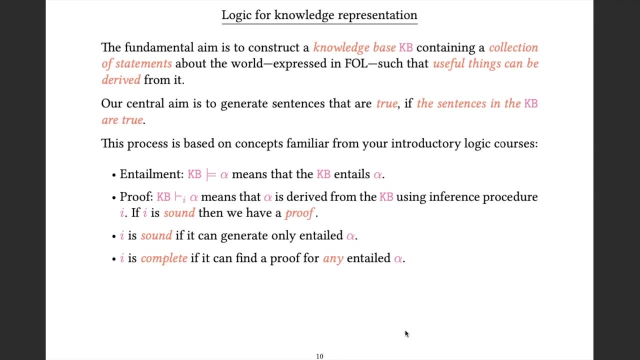 order to actually define what the function and predicate names are for your knowledge base, you need to have a proof procedure that is completely true. So if you do that in such a way that the knowledge base comes out being true, alpha will come out true as well. 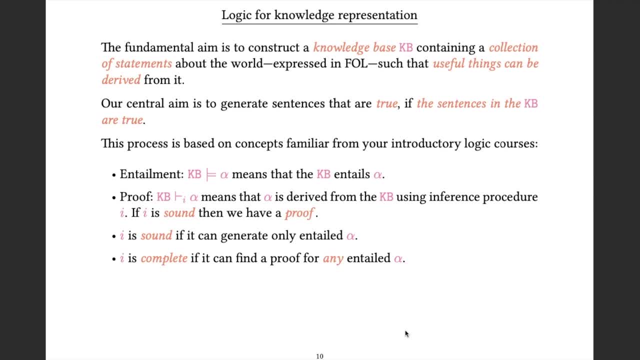 Now, clearly, you don't generally want to try and reason about all possible ways of coming up with the model, So a proof procedure is then an entirely mechanical process that just manipulates symbols that appear in the knowledge base and allows you, by a mechanical means, to prove alpha in such a way. 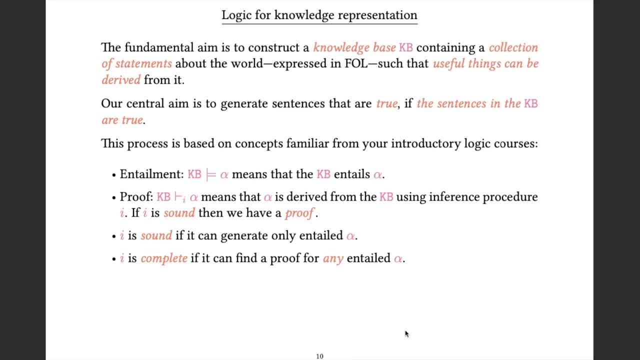 that proving alpha from the knowledge base is equivalent to saying that the knowledge base is true. When you write down formulae or statements in a knowledge base, you will inevitably use concepts that reflect the world that your agent is living in. Those will turn up, for example, as function and predicate names within your knowledge base. 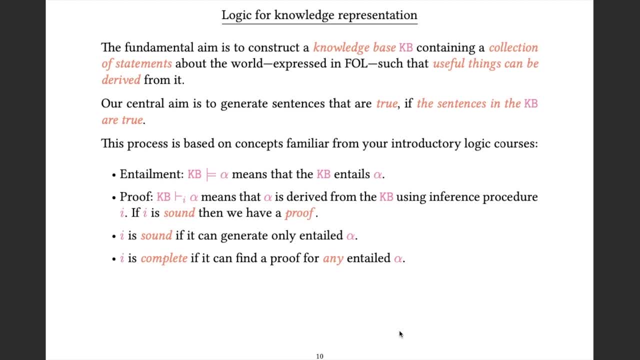 Those names have no intrinsic meaning. when you specify a model within first-order logic, You give them a meaning because you give the function names an actual function, the predicate names an actual predicate, and so on. But entailment means that no matter how you assign those predicates and functions, 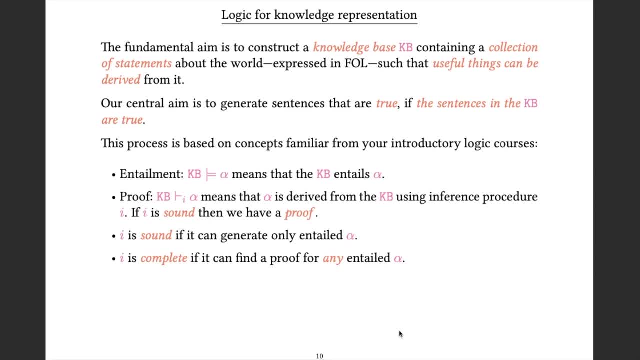 anything that makes your knowledge base true will make alpha true. Alpha is something that you're trying to infer from the knowledge base, And then the proof procedure- if it's sounding complete- is useful, because it only relies on manipulating the symbols that you are using and you don't have. 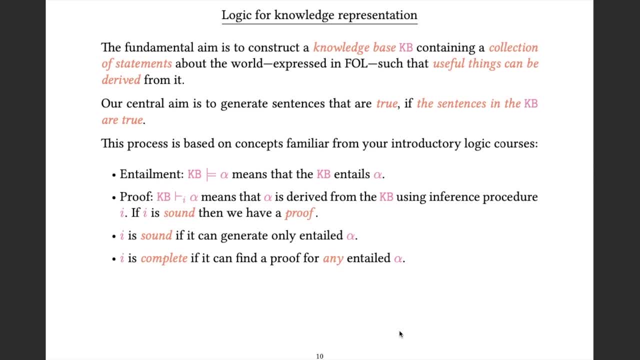 to specify a particular model in which you're interested, because all models that make the knowledge base true will make alpha, the thing you're trying to infer, true. So this is all fairly basic stuff. The key thing in terms of the process is that you will want to write down. 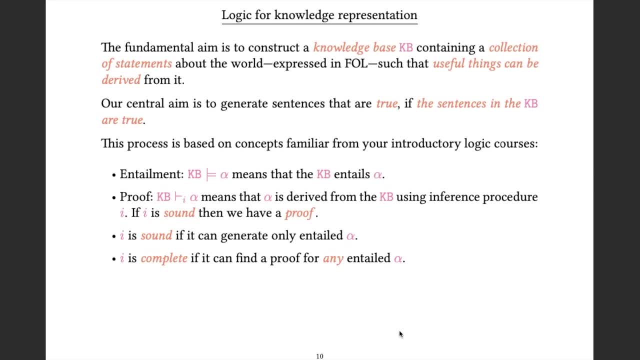 the fundamental knowledge that the agent has about the world as a bunch of first-order logical statements and those together from your knowledge base. Your inference procedure then involves setting up the thing alpha that you want to try and prove and applying the proof procedure or the inference procedure i to it, And then you know that if the things in your knowledge base are true, 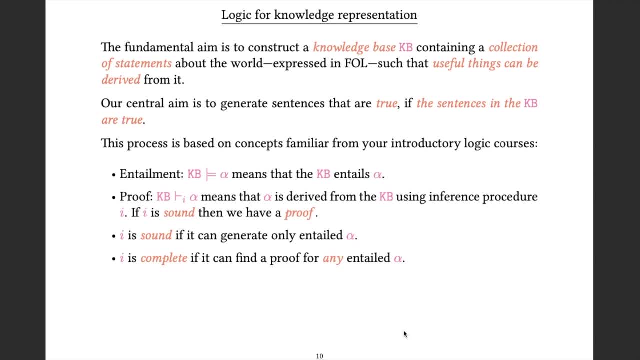 then so is the thing you're trying to infer. Once again, there is the underlying assumption here that this knowledge base is put together by a human using expertise and possibly using expert help, in order to to come up with a good description of the environment and how, actions affected, and so on. 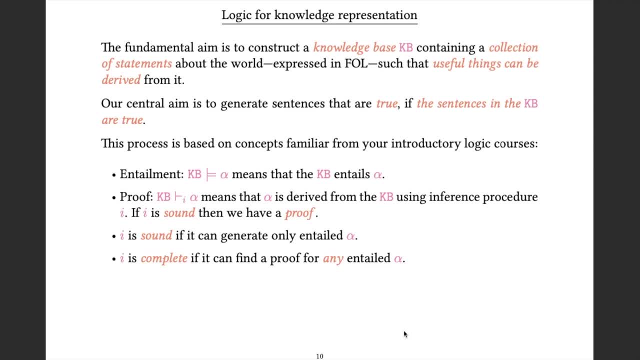 It is possible to go beyond that. So, for example, there's an area within machine learning called inductive logic programming and that allows you to infer from examples knowledge in the form of first-order logical statements. But once again, that's just a general idea of what you're trying to do. 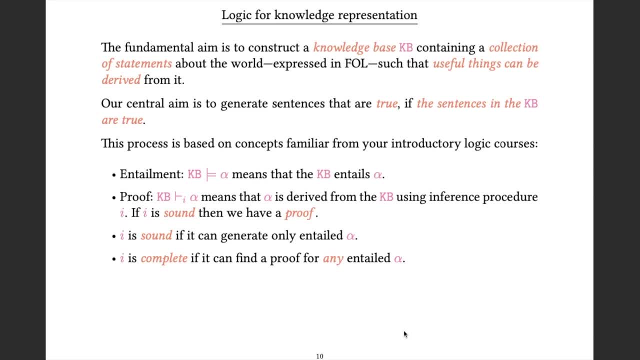 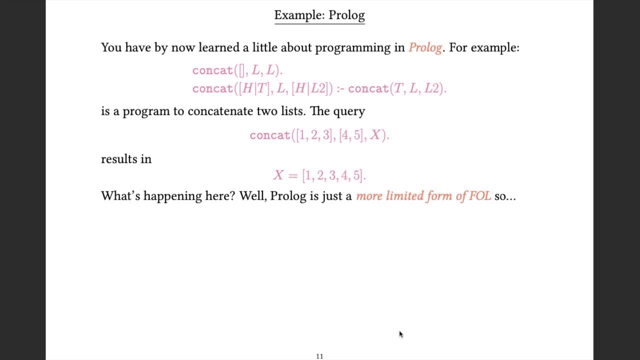 Unfortunately, I'm not going to have time to talk about that Now. somehow you've learned about this process and you've applied this process when writing prologue programs. You may, however, not have made the connection that that's what's going on, So let 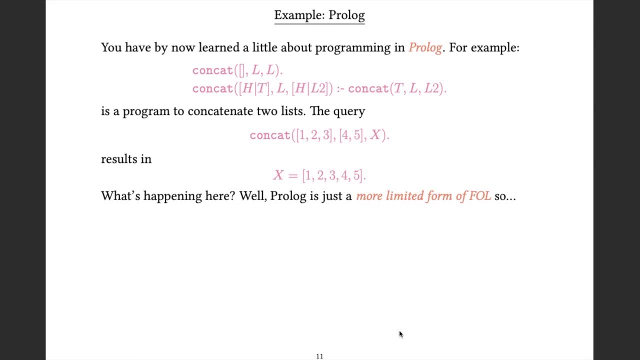 me try and make it completely clear. When you write a prologue program, you are in fact writing down a knowledge base. Your knowledge base represents some knowledge about a particular environment. In this example, I have a knowledge base that represents knowledge about the environment where 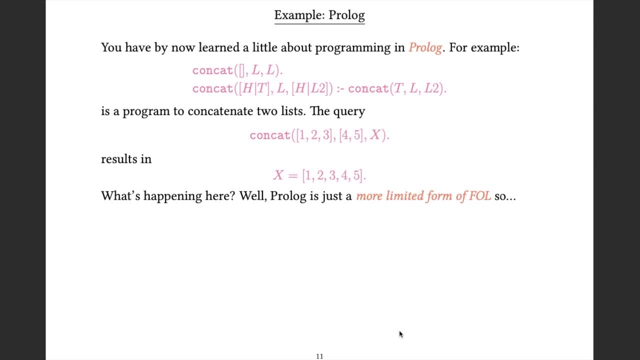 there are lists. Hopefully you can still remember your prologue from last term. This says that if I concatenate the empty list with l, I get l, and if I can concatenate t to l to get l2, then I can concatenate h cons t to l to get h cons l2.. And with that knowledge base, 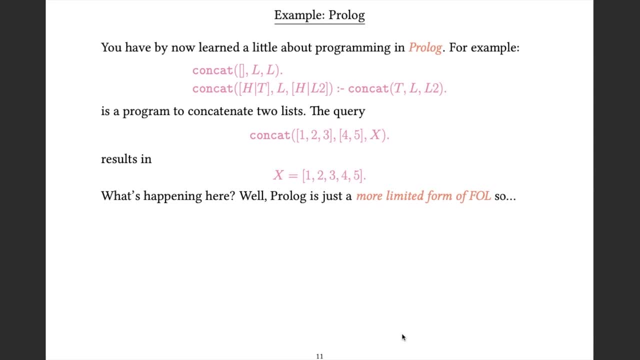 an example of an alpha that I might want to infer from this knowledge base would be something like concat: one, two, three, four, five, x, Hopefully, with the result that x is one, two, three, four, five. Now this all works because prologue is just a limited form of first-order. 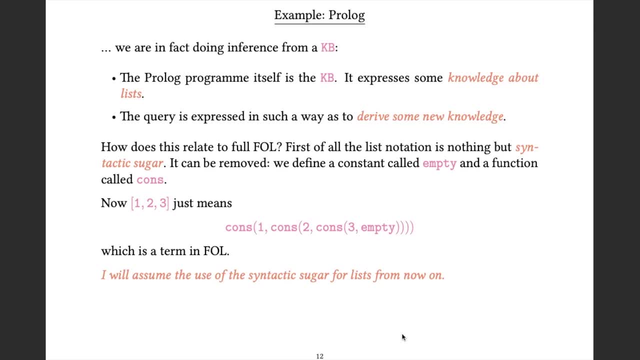 logic In a prologue program. the actual program is the knowledge base. In this case it expresses some knowledge about lists and the query is the alpha that we want to prove from that knowledge base. It's important initially just to emphasize that the list notation is just syntactic sugar. We can model lists in. 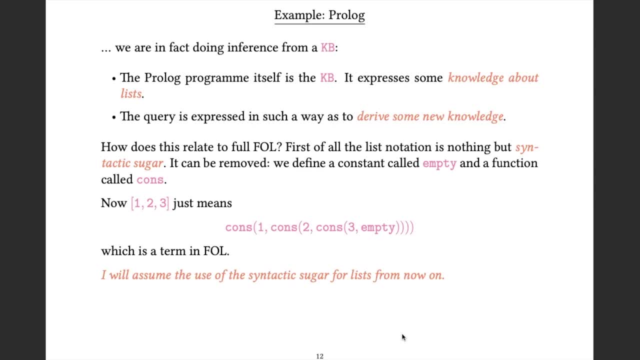 first-order logic by having a constant called empty, denoting the empty list, and a function called cons that takes two things and adds the first onto the second, the first being the head and the second being the tail. That just means that, for example, if we apply the function cons to 3 and empty, it maps to. 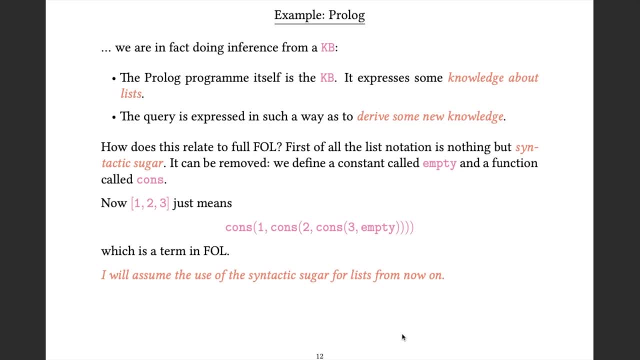 some element within the underlying universe that represents a list with 3 in it. If we then take the function cons and apply it to 2 and that element and that element, then we get an element within the universe that represents the list with 2 and 3 in it. Now I'm going to assume that we have that syntactic sugar from. 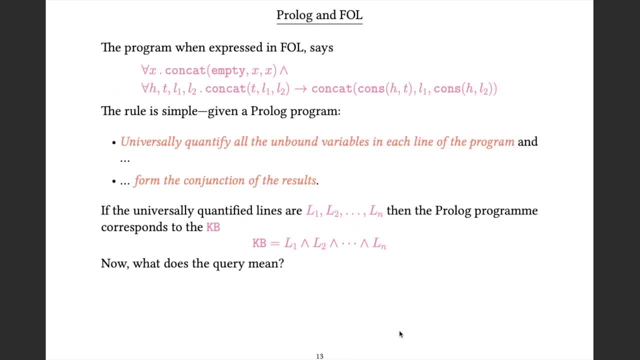 now on, If I take the prologue program and express it purely in terms of first-order logic, we get something like the following: Now, all that's happened here is that I've changed from the prologue notation to the more usual notation. I've quite cool him with the system很 잘. 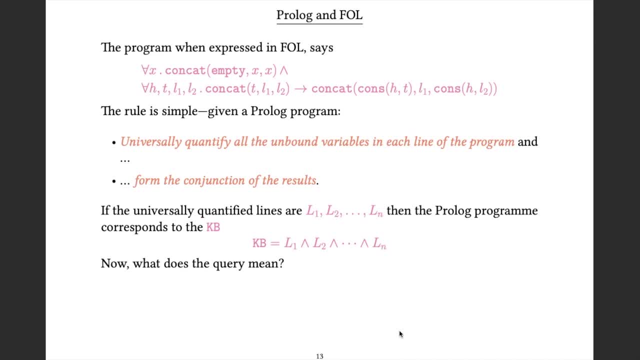 used the idea that cons' is itself a function and that empty is itself a constant and I've put back in the universal quantifiers which are implicit when you write a prologue program. Now I have the first-order logic equivalent of the prologue program For all X. concatenating empty to X gives 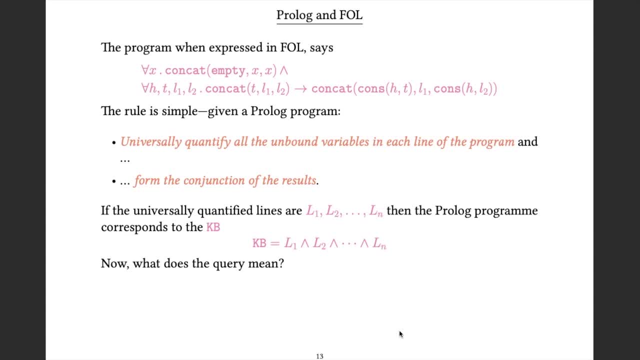 you X and for all heads, tails would be double list1s and list2s. concatenating tail to list1 to get list2 implies that you can concatenate cons ht to l1 to get cons h- l2.. In logical terms, those individual lines of the program are then just concatenated together to give you: 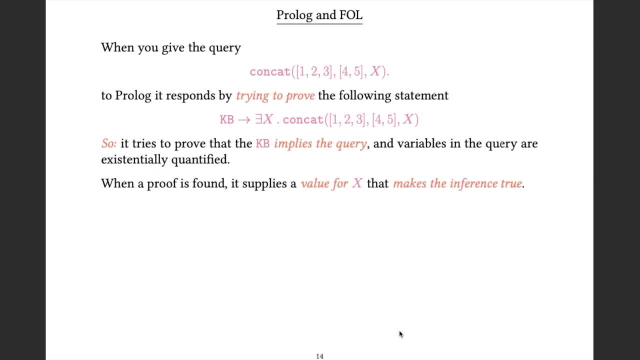 the knowledge base. Now we then want to ask what the query actually means. A query that has variable spaces in it, like x in this case, in Prolog, corresponds to an attempt to prove that your knowledge base, represented by the Prolog program, implies the query, but with an existential quantifier attached to each. 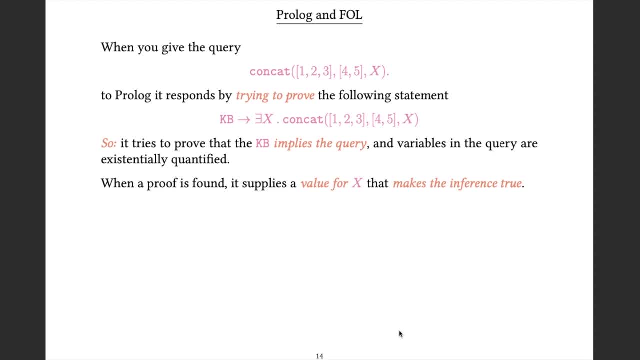 variable. that's in the query And that's what goes to your theorem. for this, Prolog is a simplified first-order logical theorem prover, which, in the case of Prolog, is a simplified first-order logical theorem prover. It's simplified because you can only have horn clauses. 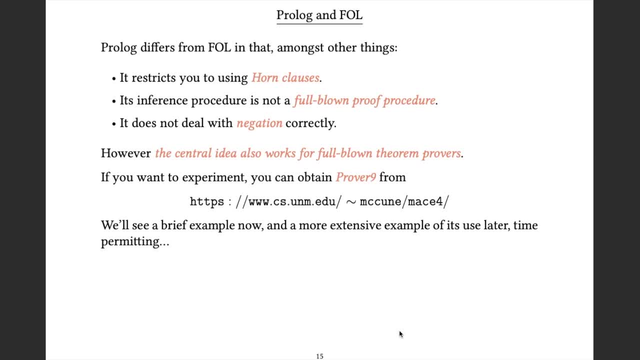 you can only have one thing on the end of your implication: it's not a foolproof procedure. it doesn't do negation correctly because it uses negation as failure and so on. But what I would like you to do, particularly for the purposes of completing the problem sheet, is download: 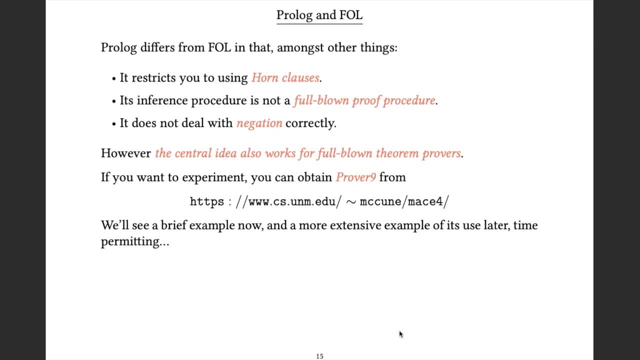 yourself a copy of Prover 9, or, if you have a preference like e or vampire or whatever, you're welcome to use another first-order theorem prover. But please do install and learn the basics of how to call one, because you'll need that for the. 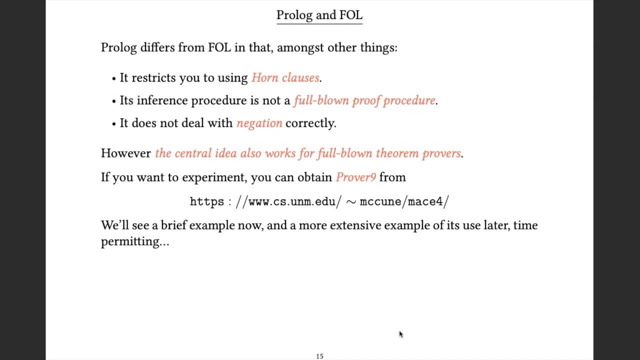 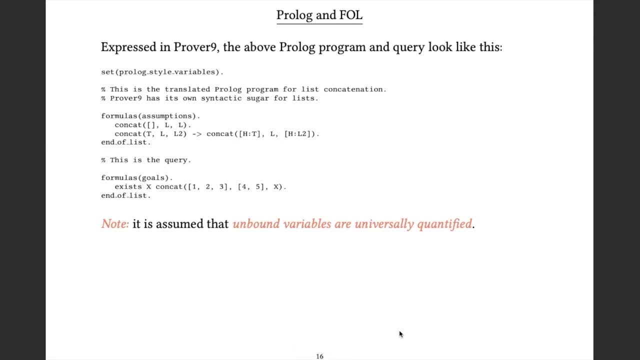 problem sheet where I want you to actually put some of the material I'm about to talk about into practice. If you're using Prover 9 as a full-blown first-order logic prover, then our initial Prolog program involving the list environment can be. 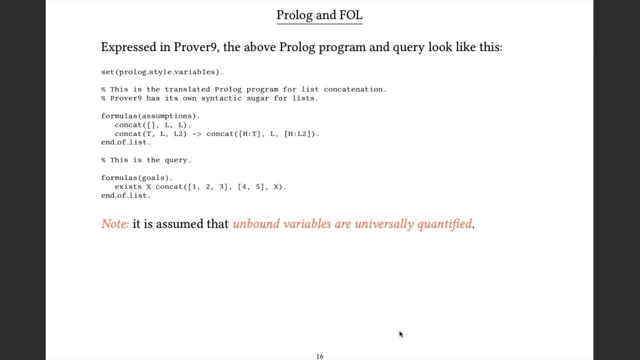 expressed as follows: Once again, unbound variables are assumed here to be universally quantified. The first line just says that we're going to use Prolog style variables, because usually Prover 9 doesn't like it if you use uppercase things for variables in the way that Prolog does. We now have a couple of 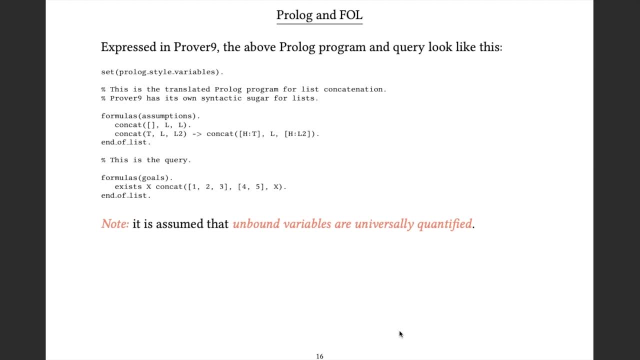 comments. Assumptions allows us to specify what the underlying assumptions are, in other words what the knowledge base is. and here we have a direct translation of the Prolog program, just using Prover 9's version of the list syntactic trigger. 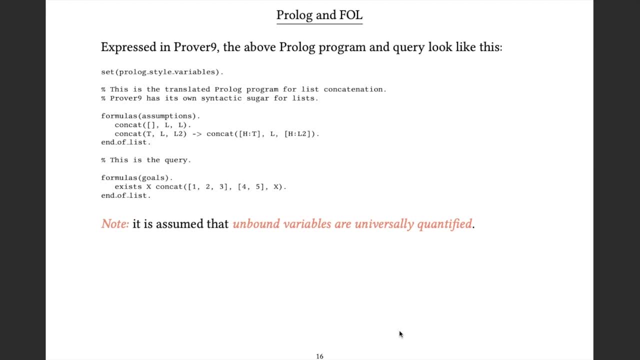 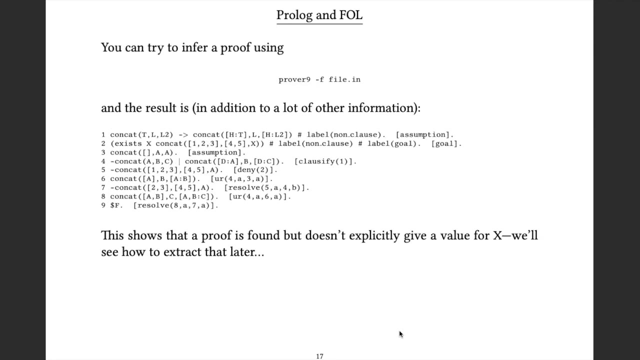 And then the query for this particular theorem, prover, goes within formulas, goals, and now we need to explicitly say that there's an existential quantifier for x. And if I put that in a file called filein, I can run Prover 9 using Prover 9 minus f with. 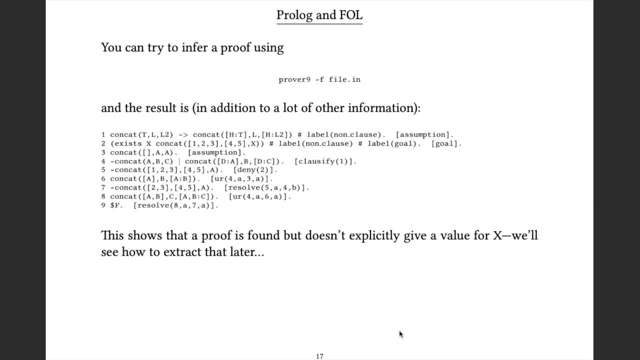 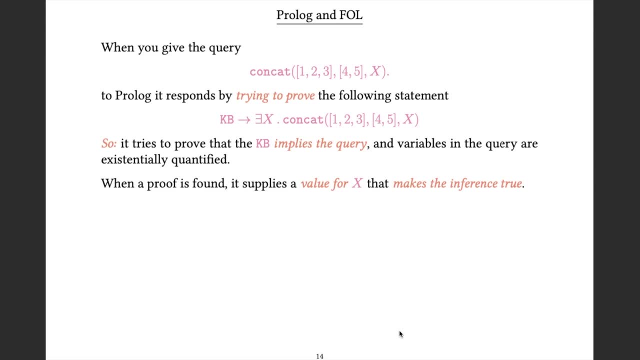 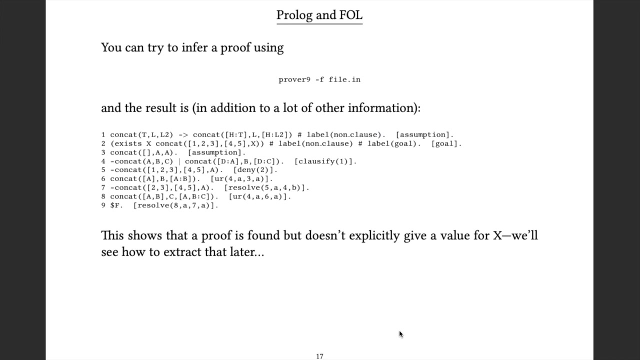 the file name and I get a whole bunch of stuff out. Essentially, what happens is it converts that whole program into the statement here that you're trying to prove, namely that the material in the knowledge base, the assumptions, implies the goal, And you can probably see by having a bit of a trawl through this.